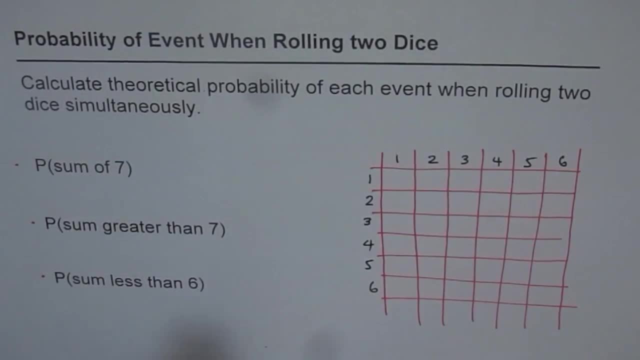 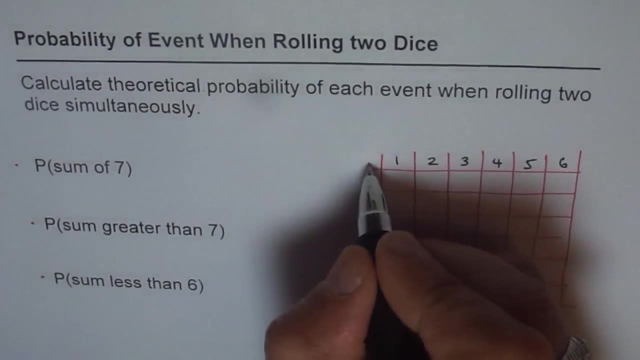 four, five and six correct. Now what operation are we doing? We're throwing the two dies there, and adding sum means add them up. So let's try to add them up. If you add these numbers, what do you get? 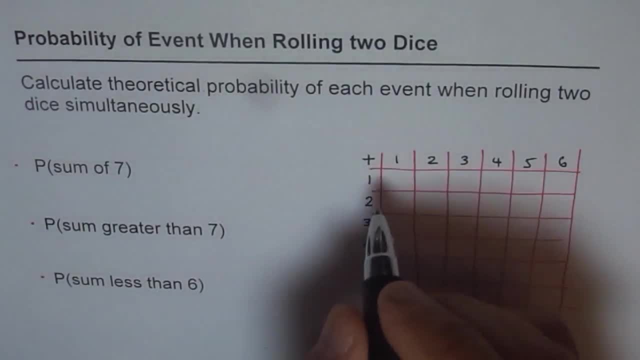 So let's add and fill up this table first. So one plus one is two now. one plus two is three, now one plus three. so we'll add one to all these numbers and fill up the first row. so we'll getting four, five, six, six. 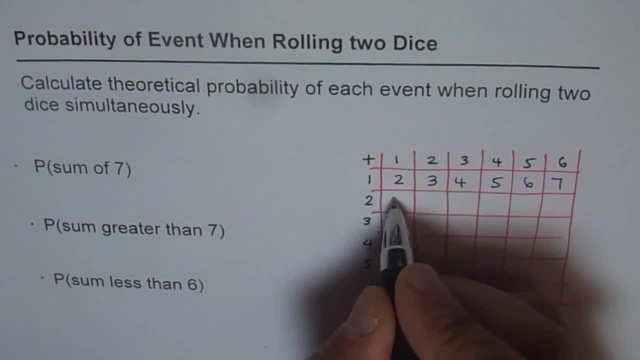 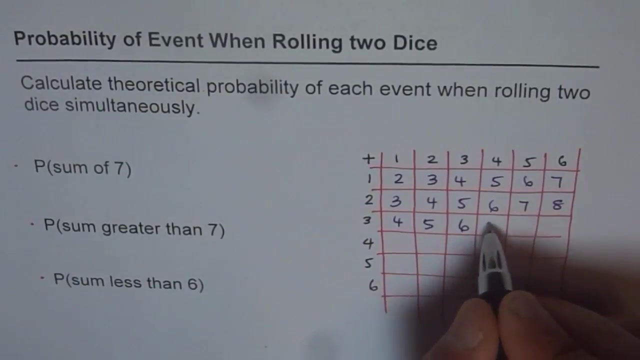 plus one is seven. Now let's add two to this, so we get two plus one, three, four, five, six, seven, eight. let's add three to this series, So it starts with three plus one, four, and plus two is five, six, seven, eight, nine. 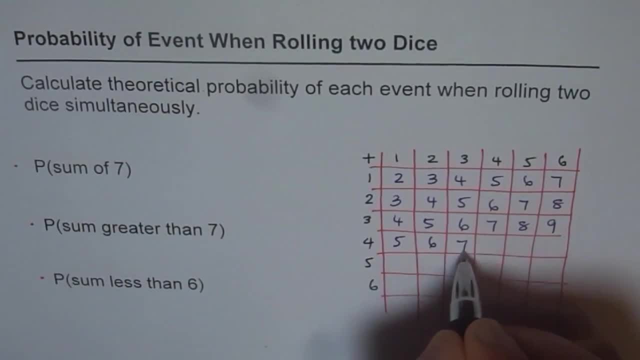 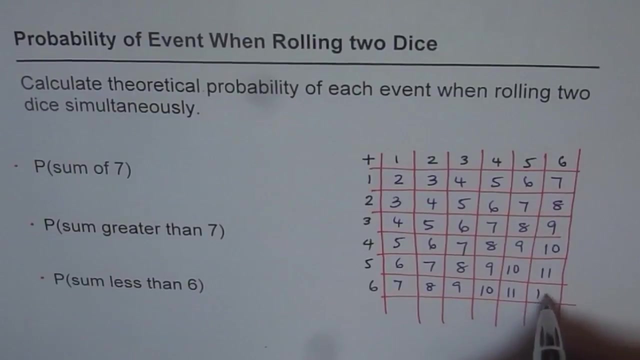 Let's continue. four plus one, five, six, seven, eight, nine, ten. Five plus one is six, and then seven, eight, nine, ten, eleven. Six plus one is seven, and we get eight, nine, ten, eleven and twelve. 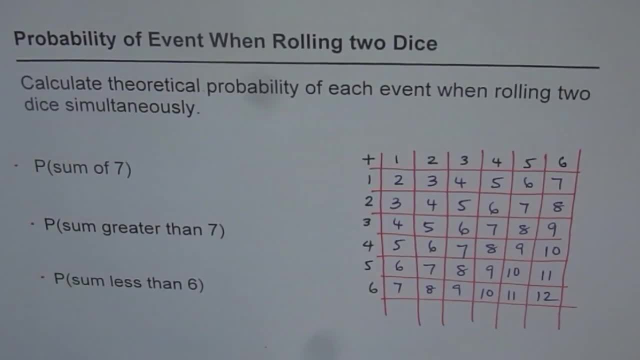 So that is kind of the matrix which you get right. So when you add the combination of roll from the first die and with the other die, then the total is given here right in the center right. So for example, if you roll from the first as number three and from the second as number, 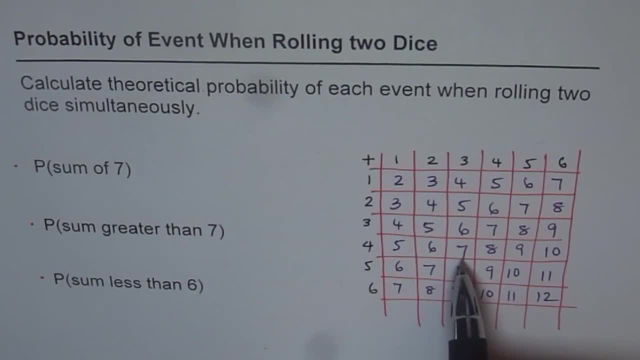 four, their sum is seven, correct. That is how we have to see and observe this right Now in this particular question. we have to find the whole number, Find the probability when the sum of five for the sum of well, in this particular thing, 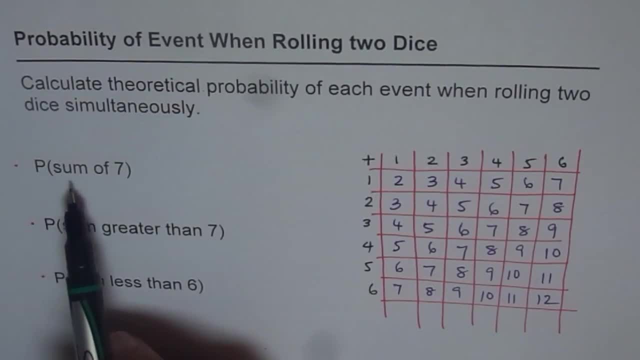 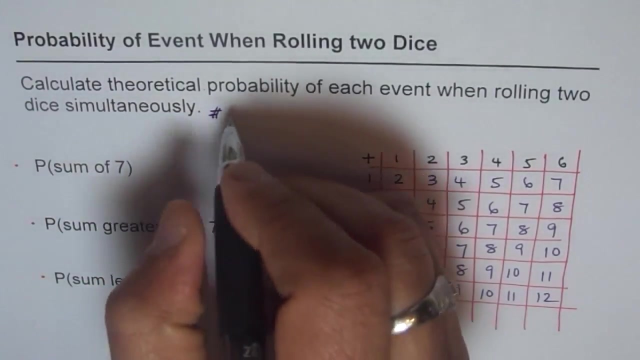 the first one is: find the probability for the sum of seven right. So first is: how many possible outcomes are there? You have to figure out how many possible outcomes are there. That means we have to answer the question: number of all possible outcomes. 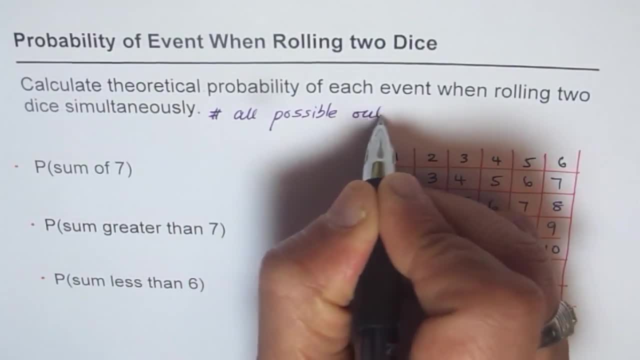 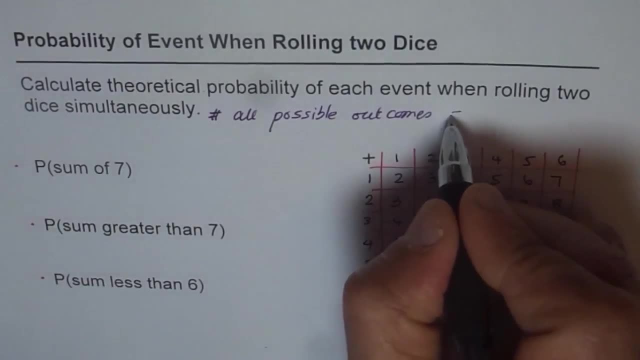 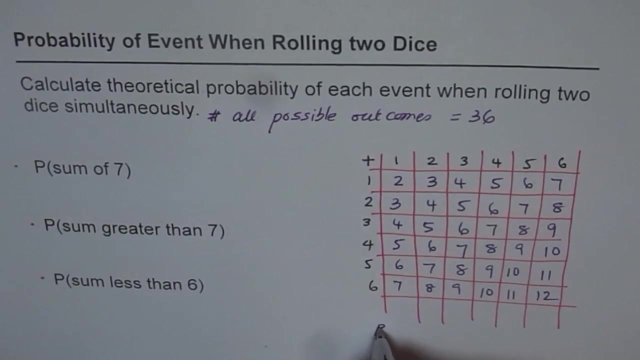 Right Outcomes, because that goes in denominator. It is six times six. If you count these, there will be thirty-six in all right, There are thirty-six, So that is in the denominator. So probability, which we are trying to figure out, for anything will be equals to here possible. 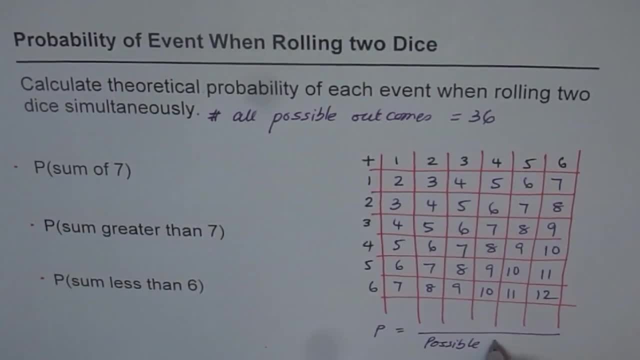 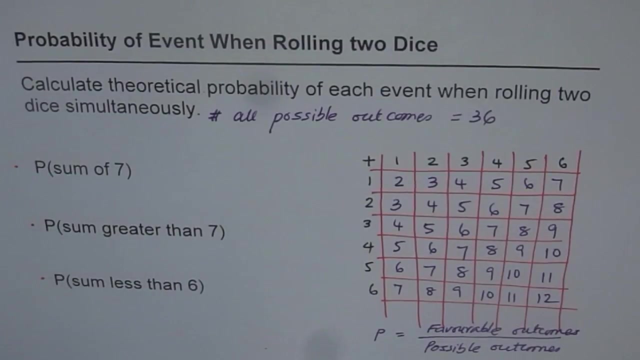 outcomes right. Total possible outcomes right. Yeah, For this numerator we have got favorable outcomes right. Their ratio is going to give us the probability answer. that is what we have right. Sum of seven. So we already have a table and you can see where do we get seven. 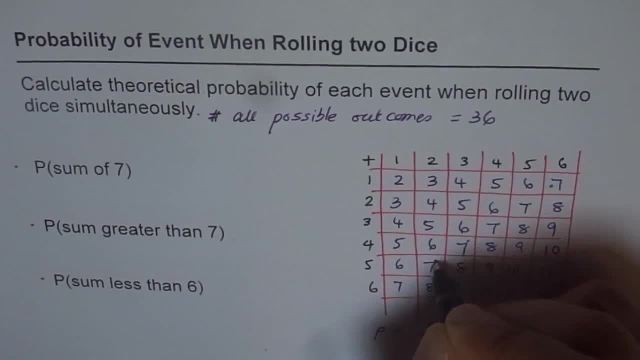 So we get sevens here. Do you see that? These are our sevens? Do you see that? How many are these? One, two, three, four, five, six, right? So that is how many times you get seven. 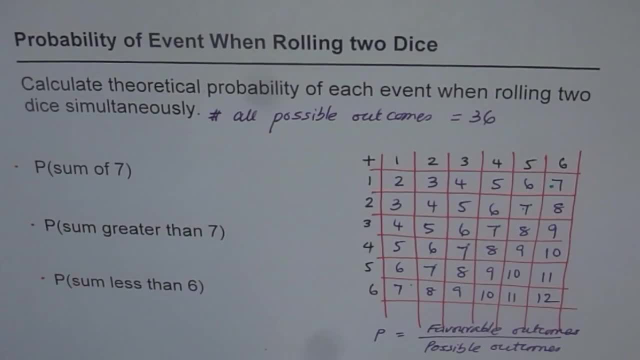 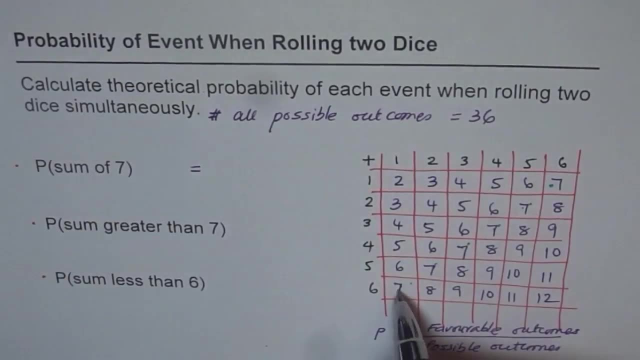 Do you see that you get 7 in this particular thing. So sum of 7, the probability is equals to 1,, 2,, 3,, 4,, 5,, 6, right? So 6 times you can get 7 in this particular matrix, or total possibilities. 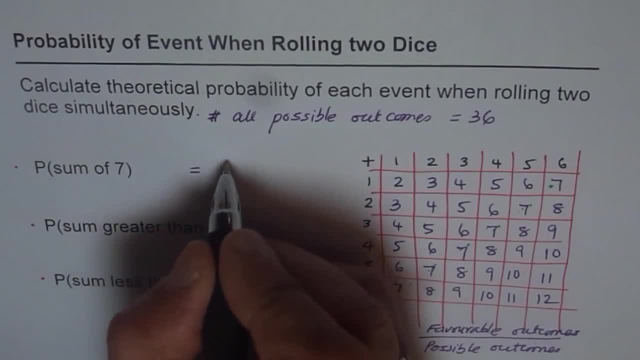 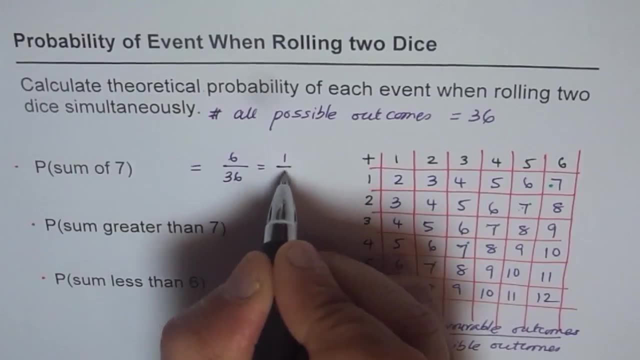 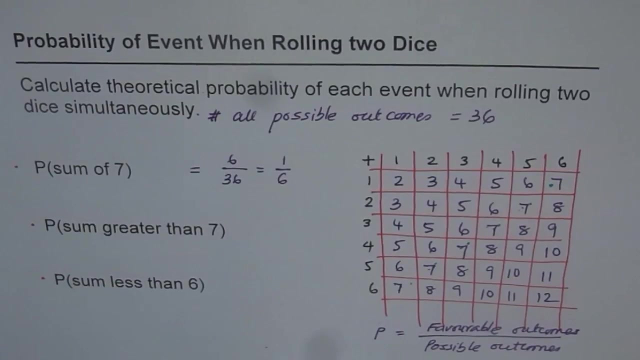 So the possibility of getting 7 is 6 over 36, which is total number of outcomes. Rather, 1 out of 6 times 6 is 36 can be written as 1 out of 6.. So that is the probability of getting sum of 7, correct. 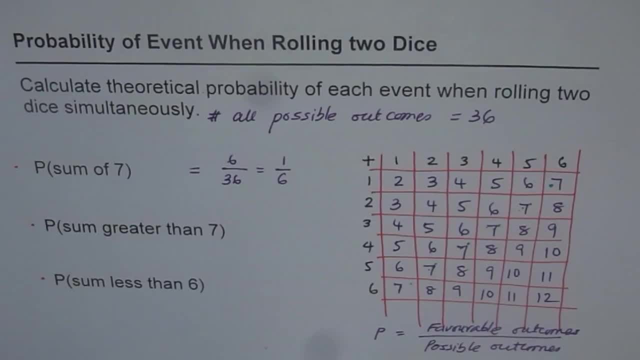 Now what is the probability of getting a sum greater than 7? That is what we have to figure out. So the numbers greater than 7 are given here. So they are right here: 8, 9.. These are the numbers greater than 7.. 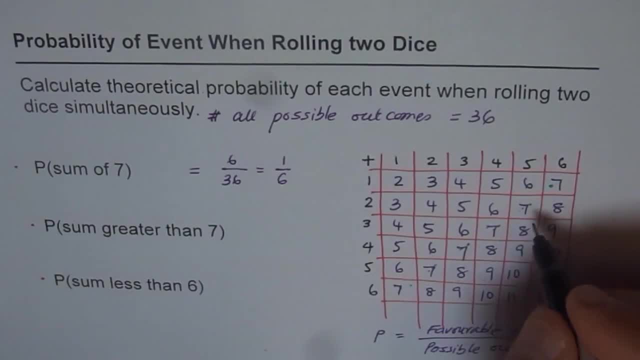 So let me mark these numbers for you And then we'll count them right. So the numbers greater than 7 are given for us in this list. These are all the numbers which are greater than 7 when you add right. So how many are these? 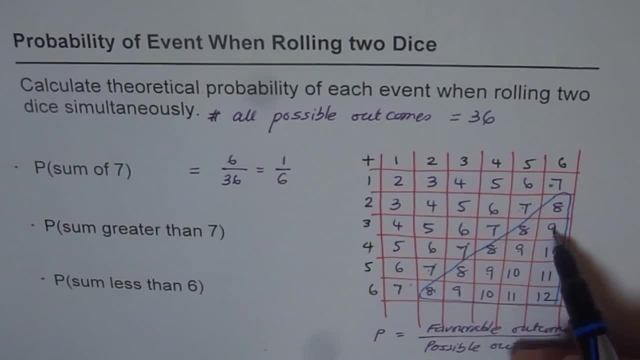 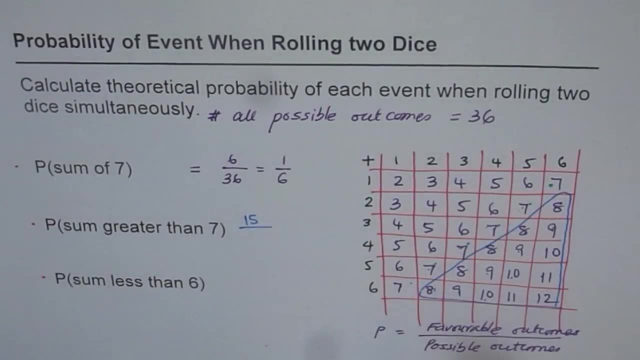 1,, 2,, 3,, 4,, 5,, 6,, 7,, 8,, 9,, 10,, 11,, 12,, 13,, 14, 15.. So we get answer here is 15 out of total of 36, right. 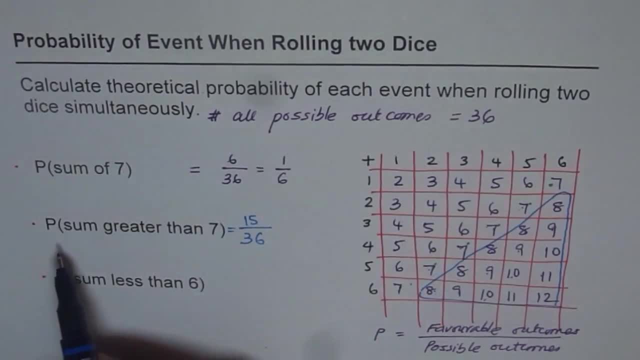 15 out of 36.. So that is the probability When sum is going to be greater than 7.. I hope you understand that. And the next one is probability when sum is less than 6.. Now, which are these numbers Where the sum is less than 6.. 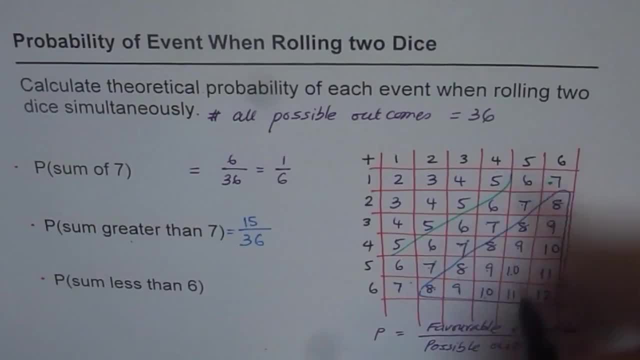 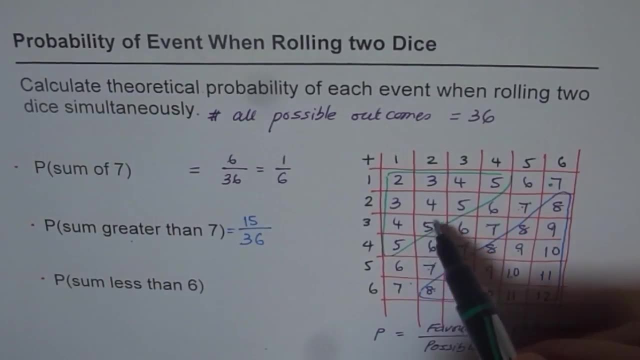 So that is the numbers here: 5 and lesser than 5.. And that is this set of numbers. Do you see that? Let's count how many of these? 1,, 2,, 3,, 4,, 5,, 6,, 7,, 8,, 9, and 1.. 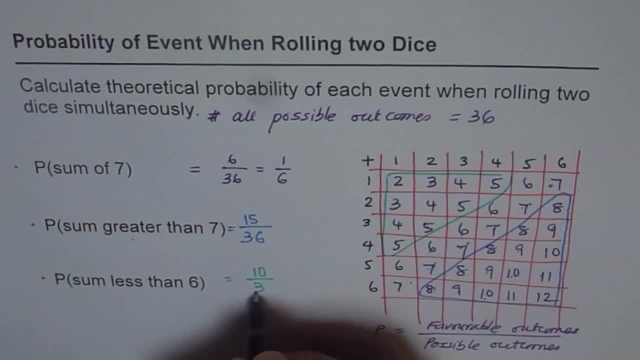 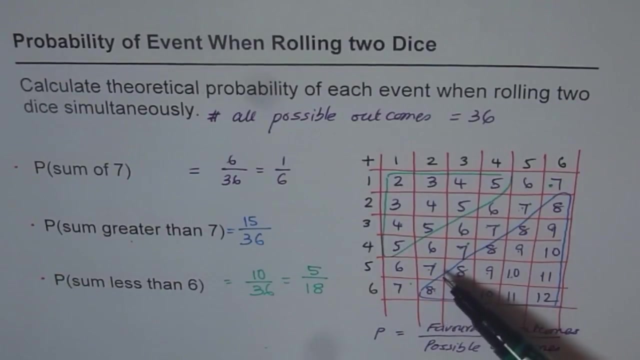 10.. So we get this as 10 over 36. Which you can simplify dividing both by 2.. So 5 over 18, right. So that is the probability You can see. the maximum probability is amongst these for getting numbers more than 7, right. 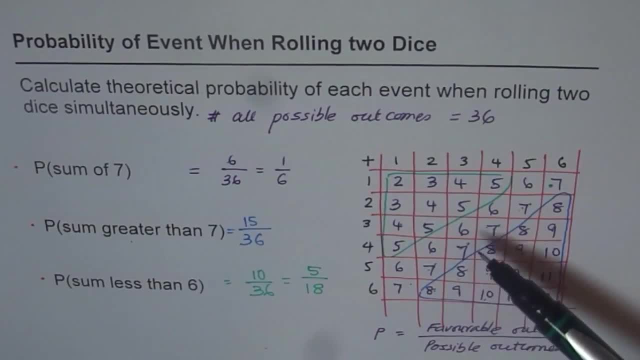 And less than 7, rather less than 6, is 5 out of 8.. Correct, So these are the different probabilities When you roll two dice at the same time. I hope you understand the concept. The critical issue here is make a matrix or a table of values like this: 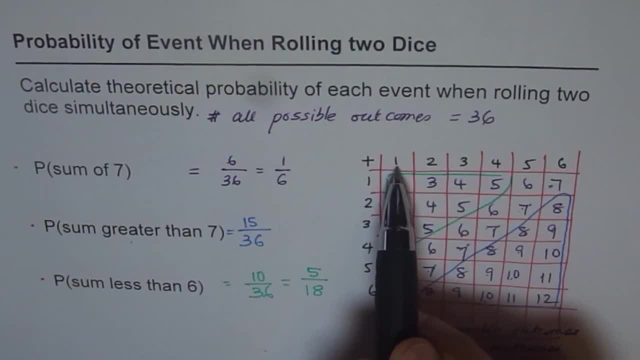 Imagine the one dice numbers are or the outcomes are written in one column And the other row has list of other six outcomes. Add them and fill up your table. Once you do that, you get total number of outcomes. Here the total number of outcomes are: 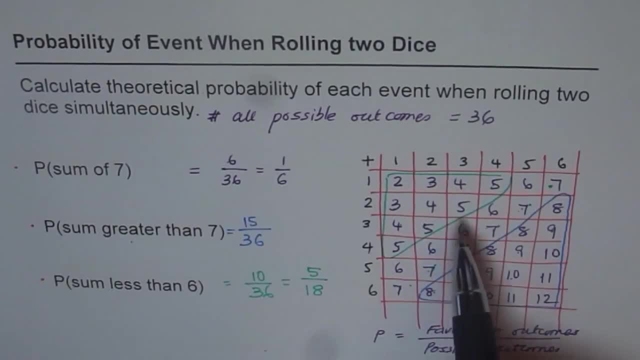 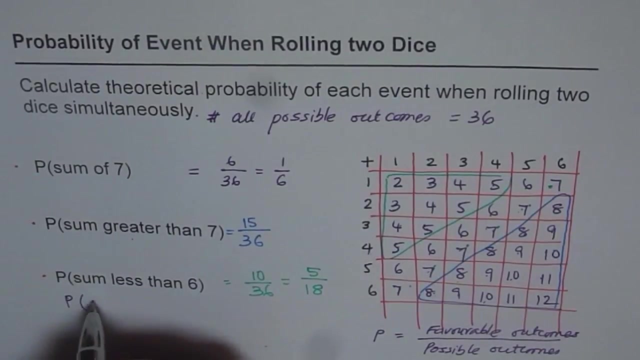 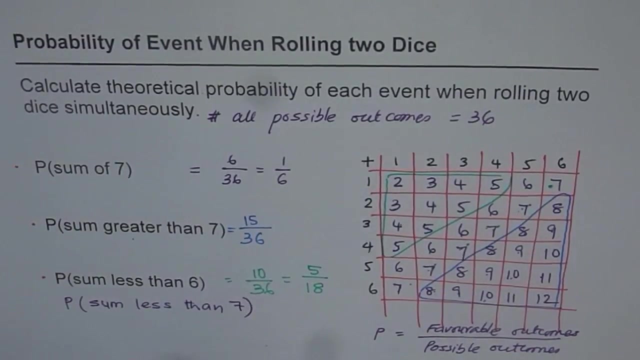 36.. Out of them, count the favorable for each. Write down the favorable in the numerator and total in the denominator. The ratio gives you the probability, correct? Now let me give you a question. So that is, figure out probability for some less than 7, right? 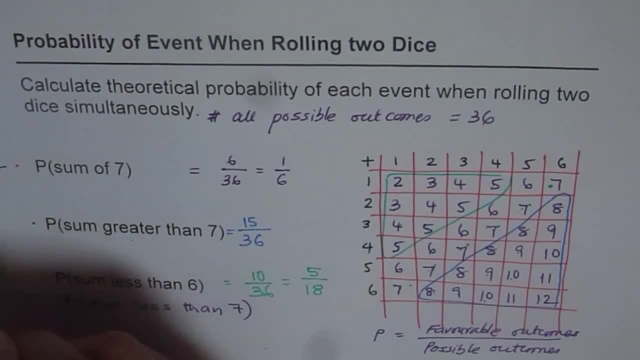 And also check with your answer. if you add this, this and this, What do you get? and why? Explain your answer? OK, so that is the question for you to work on. I hope the concept is clear. We'll do one more, and this time we will check the product when we throw the dice. OK, thank you.